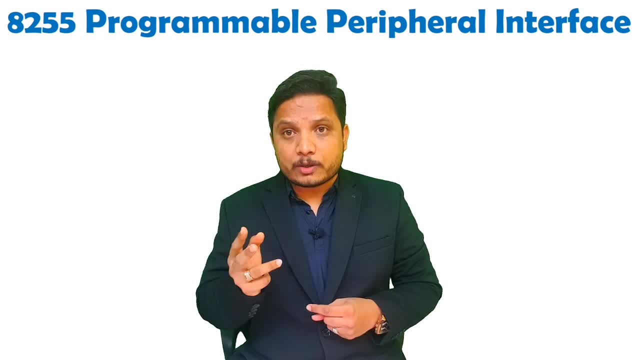 we are having three 8 bits ports and those three 8 bit ports that we can interface it with other peripheral right. So here our agenda is to increase Interfacing capacity by using 8255.. So here in this video I'll be going to explain you. 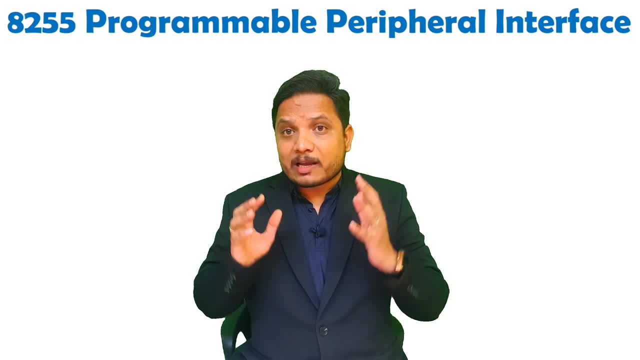 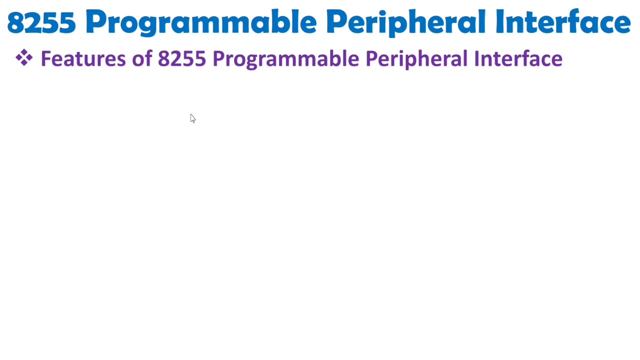 how 8255 IC is working, along with its block diagram as well, as I'll be going to explain you features of 8255.. So let us see first how many features are there with 8255 IC. So when we talk about 8255 programmable peripheral interface, IC's features. 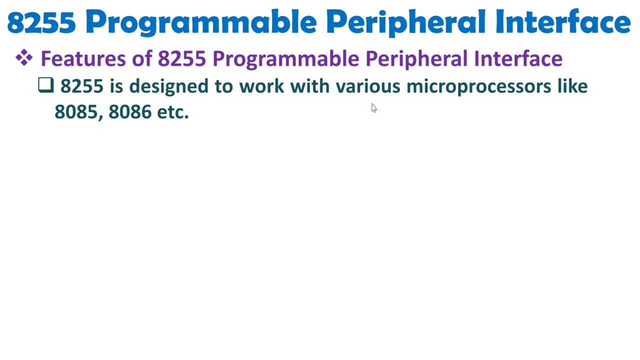 then you should know, my dear students, it is designed to work with various microprocessors like a 8085 and 8086.. Here our basic agenda is to increase capacity of interface in terms of input output interface. here, 8255 is having 3 8bits ports and these 3 8bits ports 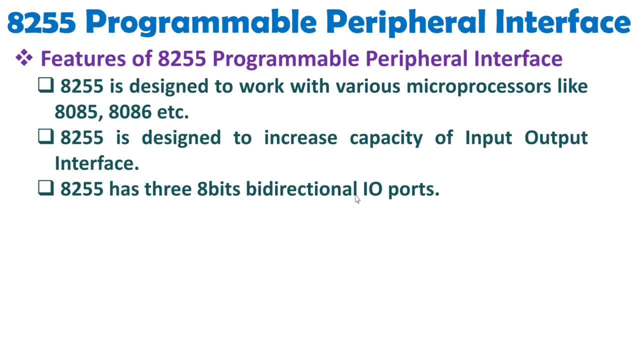 those are bidirectional IO ports, So we can use those ports as input as well as output. Here 8255 works with three IO modes, and those three IO modes are simple IO mode in which simply we just provide input and output operation. Secondly, we have handshake IO mode in which we provide 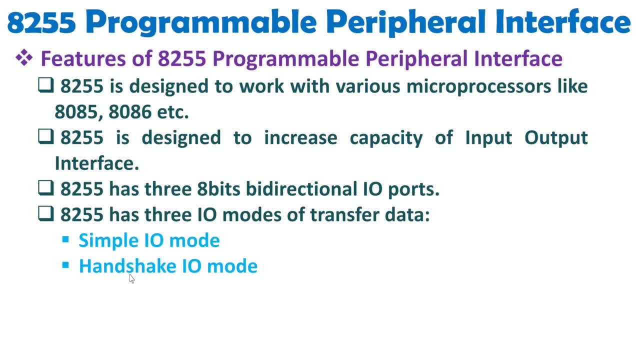 transfer of data along with handshake. Handshake means initialization. that will be done and in that you can have transfer of data Here. third mode is bidirectional handshake IO mode. So in bidirectional handshake IO mode we can have transfer of data from microprocessor to 8255, as. 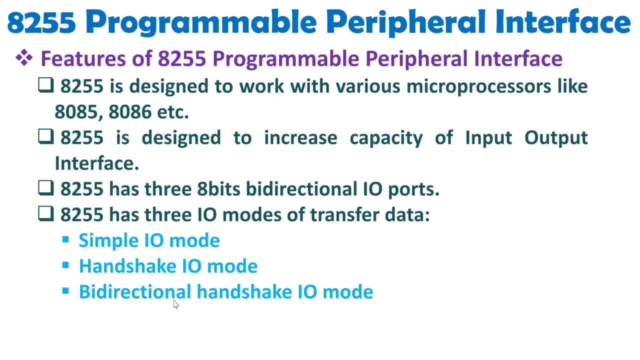 well as from 8255 to microprocessor, right. So bidirectional handshake, IO mode, that is there. Now, why there is a need of handshake, You should know, my dear students, with 8255, we don't have clock integrated inside. 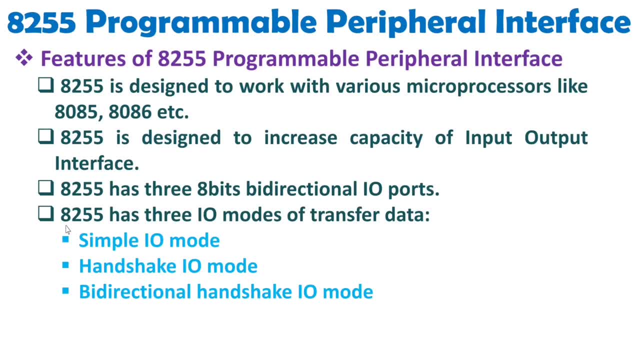 So here, before you start with communication of transfer of data, you will have to provide control signals which will identify that how data exchange should be done. So for that handshake is required, right, If you just want to simply output the data or you just want to take simply. 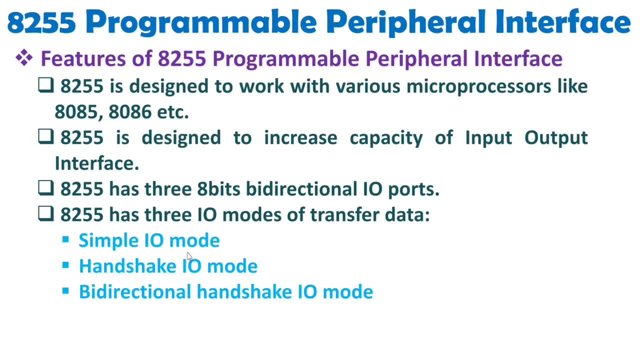 data input. in that case we can work with simple IO mode. But when you want to exchange the data at a time, initialization of exchange change of data should be done. That is referred as handshake. So simple handshake means either input handshake or output handshake. That mode is available as well as bidirectional handshake IO. 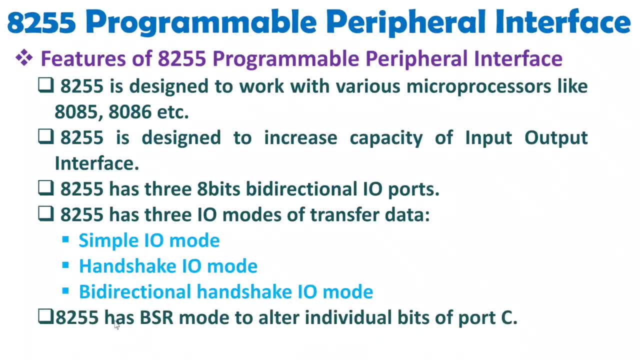 mode is available, My dear students here. 8255 has BSR mode, bit set, reset mode in which single bits can be altered, and that is possible at port C. So in coming videos I'll explain you how all these modes are operated at 8255, as well as how we can operate with BSR mode. Let us see first how block. 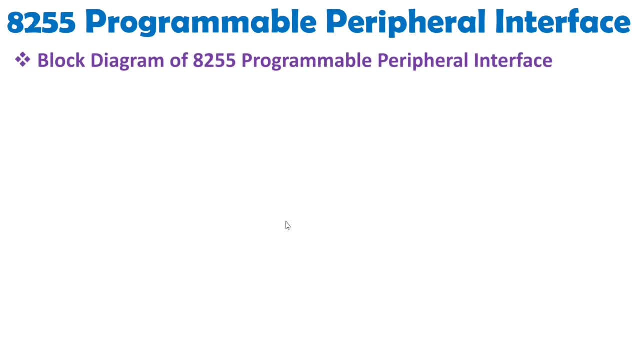 diagram is there with 8255.. So when we talk about block diagram, as I have said, it is having three, 8 bits port. You see port A, port B and port C. Port C is bisected into two nibbles, upper nibble. 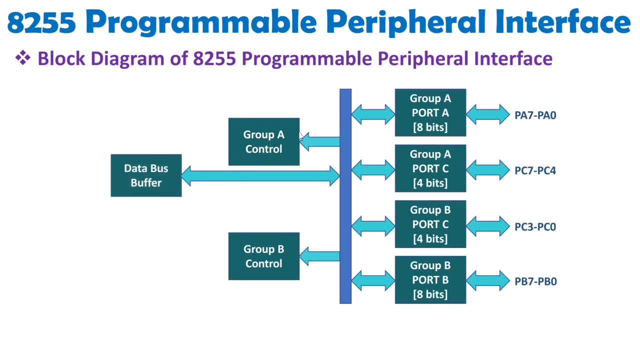 and lower nibble. Here group A that is connected with port A and upper nibble of port C and group B that is connected with port B and lower nibble of port C. Here data bus buffer is connected with system bus of D0 to D7.. Read- write logic is there with read bar, write bar A0, A1, reset and chip. 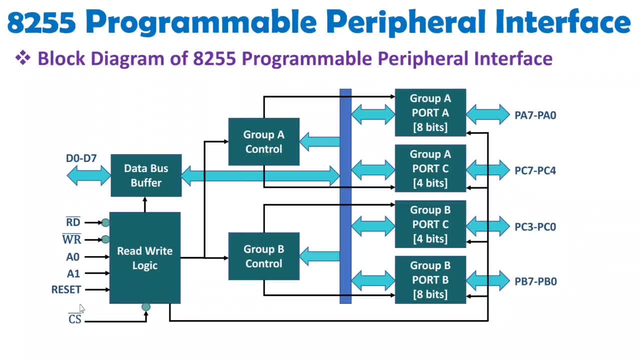 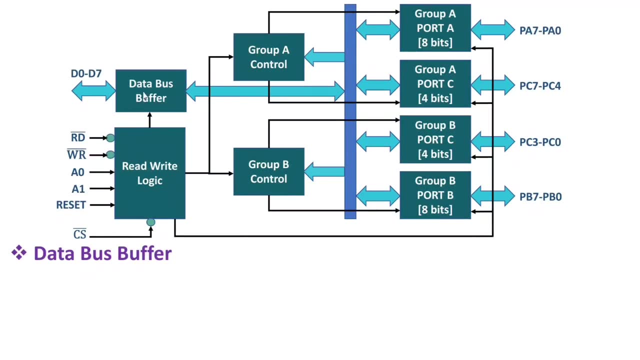 select terminals. Now, my dear students, what I'll do is I'll explain you this complete block diagram, step by step, in great details. So let us try to understand. first, data bus buffer. So when we talk about data bus buffer, you can see here: data bus buffer is there, It is. 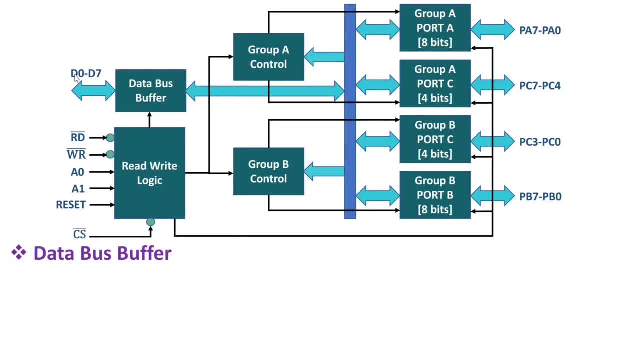 having bidirectional D0 to D7 bits which are interfaced here. So you should know, my dear students, microprocessor is having system data bus that is interfaced over here, right, And it is bidirectional. Why? The reason is, via this data bus, we will be transferring data to this port A. 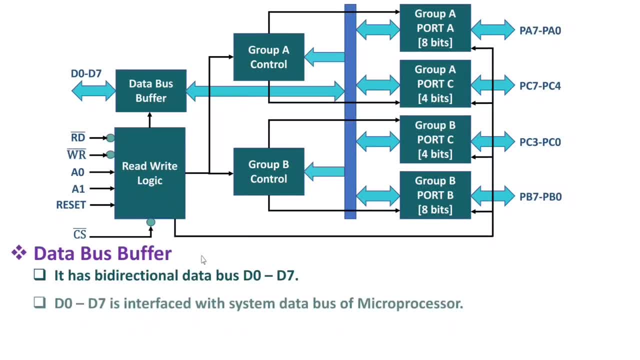 port B and port C. So here this D0 to D7 that is interfaced with system data bus of microprocessor. right Now let us try to understand first what is read. write control logic block over here So you can observe. here read: 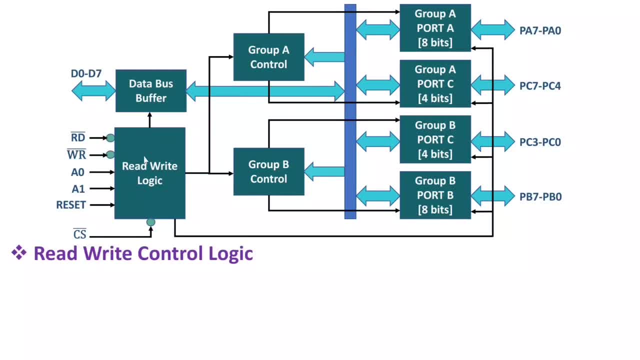 write control logic block. is there Now with this read- write control logic block? how many terminals are there: Read bar, write bar A0, A1, reset and chip select. I'll explain you all these terminals: See, read and write. those are active. low signal, That is to read. 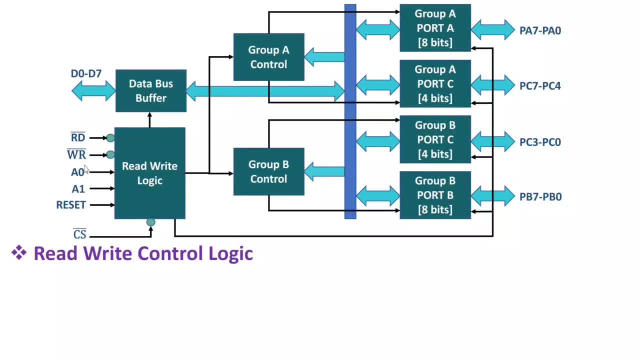 write and write. So read and write. those are active low signal. That is to read and write. So here, microprocessor that will give commands over here, right, Microprocessor's read bar that is connected over here. Microprocessor's write bar that is connected over here. It may be memory. 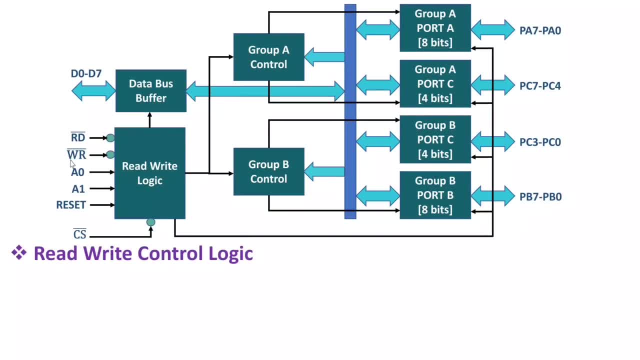 read bar. It may be memory write bar. That depends how this IC is interfaced with 8085.. If 8085 is working with memory mapped IO, in that case memory read and memory write is connected here. If 8085 is working with IO mapped IO, in that case IO read bar and IO. 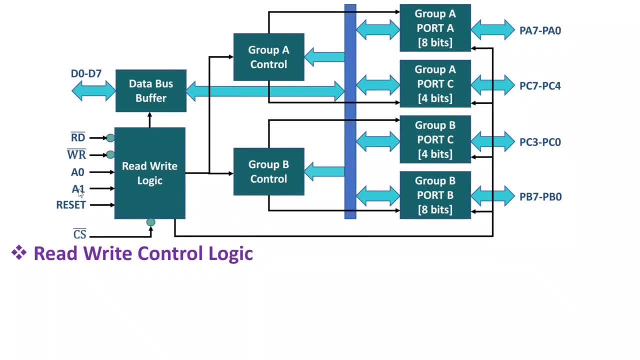 write bar will be connected here. This A0 and A1, that is to select this port, port A, port B and port C as well as that is to select control word And control word will justify in which mode this 8255 is functioning. This reset terminal that will be connected with reset out of 8085.. So 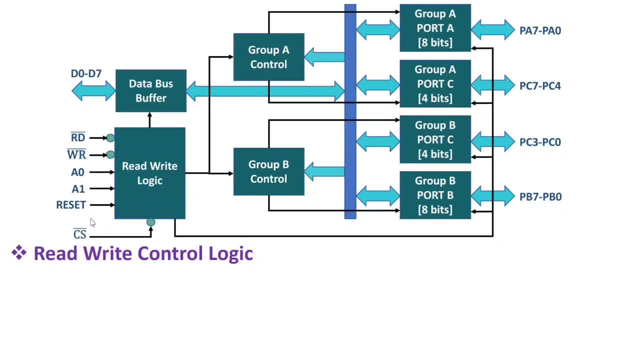 8085 can reset out of 8085.. So 8085 can reset out of 8085.. So 8085 can reset out of 8085.. So 8085 is working properly. Now let us move on to the next step, which is this is we need: 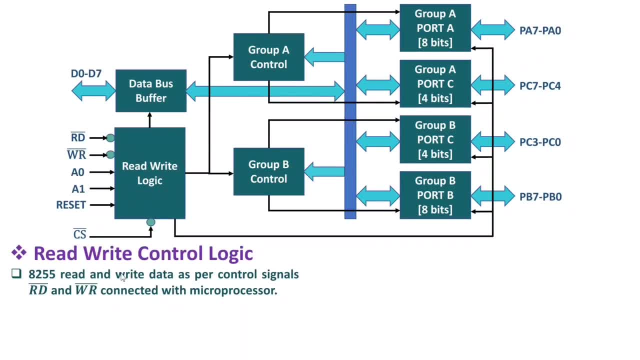 to reset this 8255.. And this chip select. that is active low signal, that is to select this chip of 8255.. So 8255 is having read write data control signal which are active low control signal Here reset will reset this 8255, A1 and A0, that is use to select neglect. 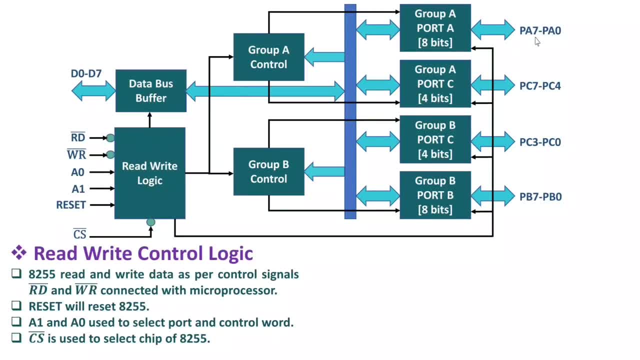 correct this: A0 and A1. that will select port A, port B and port C. So here for that. first of all, you should know chip select. that should be 0.. Once chip select is 0, as it is active low, you can operate with 8255.. If it is 1, 8255 is not selected. Now you need to see A1 and A0. If it is. 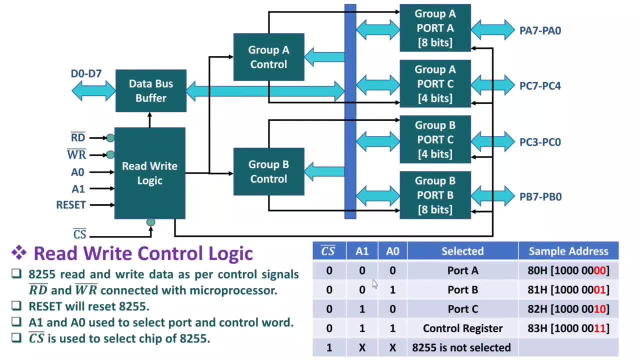 0: 0, port A will get selected. If it is 0: 1, port B will get selected and if it is 1: 0, port C will get selected. So you see here port A, port B and port C. that selection is been depending on A1 and 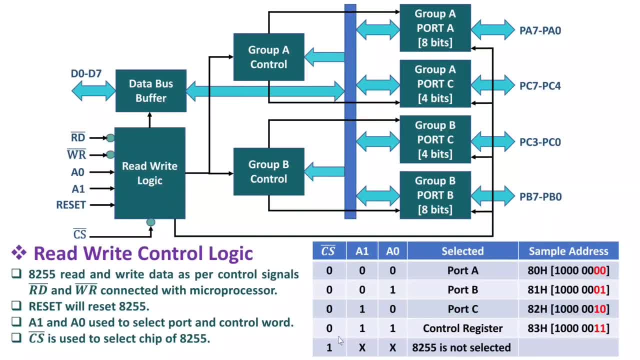 A0, these two lines right, And if it is 1: 1, then microprocessor can load control resistor over here and control resistor will justify operation of all these ports. There are total four modes available with IO operation that I'll explain you in later video. 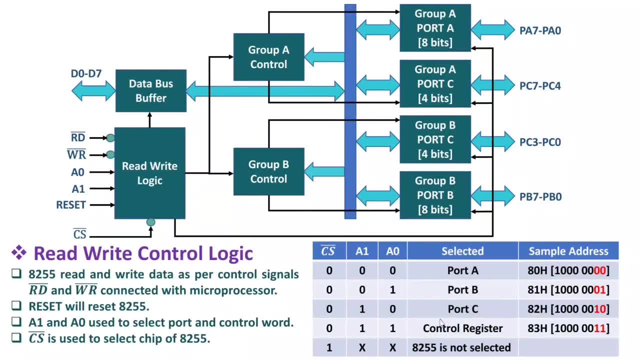 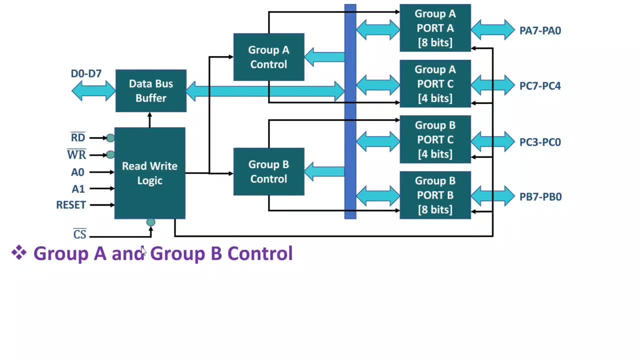 how it works. It is been controlled right. But just consider when A1, A0, that is 1- 1 control resistor will get selected and over D0 to D7 we can load control resistor over here right Now. my dear students, let us try to understand group A and group B control. Group A control is connected with port A. 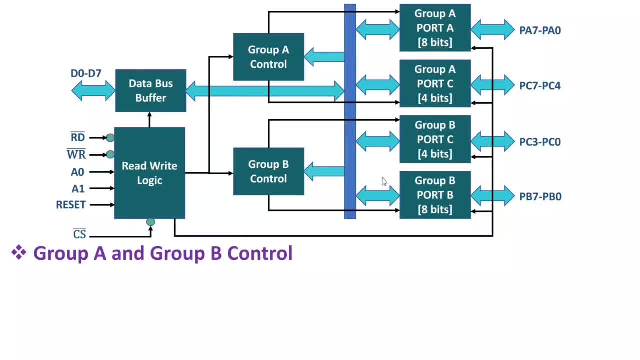 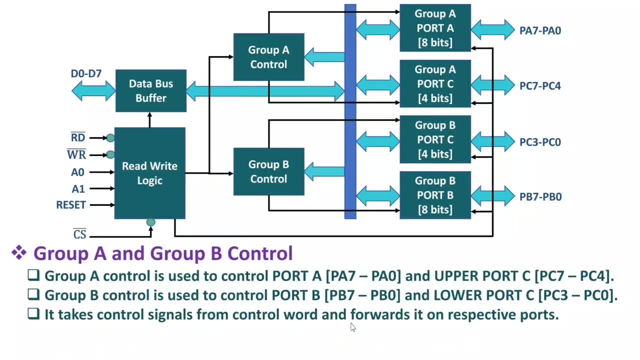 and upper nibble of port C and group B that is been controlling port B and lower nibble of port C right. So that is to have a control resistor that is selected and over D0 to D7 we can load control resistor over here right now. in point A Now we are getting control receptor and over D0. 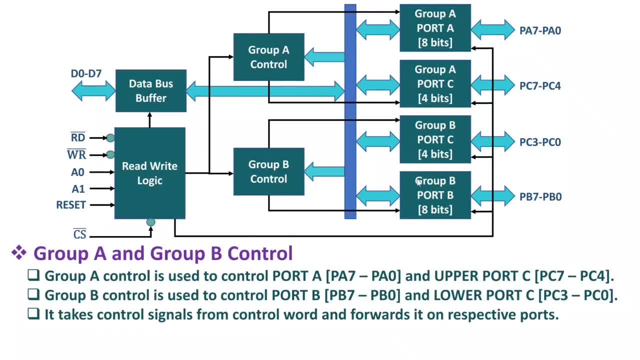 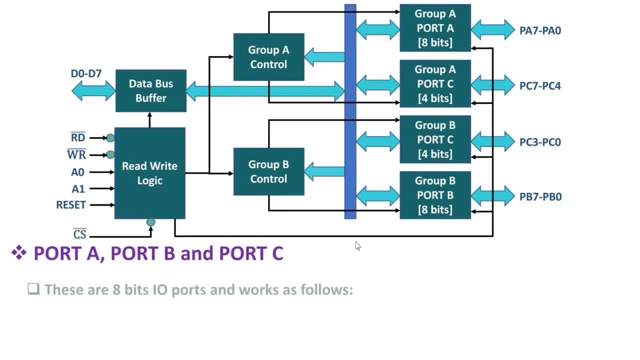 we can only have a control resistor over A1, c and over D0, D7, which is spot to a controlling of those sports right here. it takes control signal from control code word and forward it to respective port. so whatever control word is there, based on that it will be providing control to all this sports right now. my 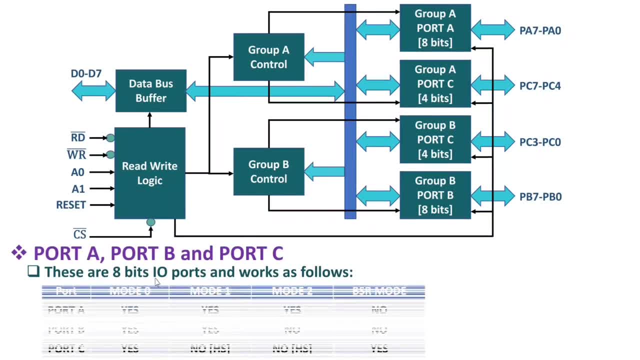 dear students, I'll explain you various modes. So let us try to understand how all those ports are working with different modes. So here, port A that is working with mode 0, mode 1 and mode 2.. Port C that we use it for handshaking and BSR mode: only Right, You should know this. Port A and port.